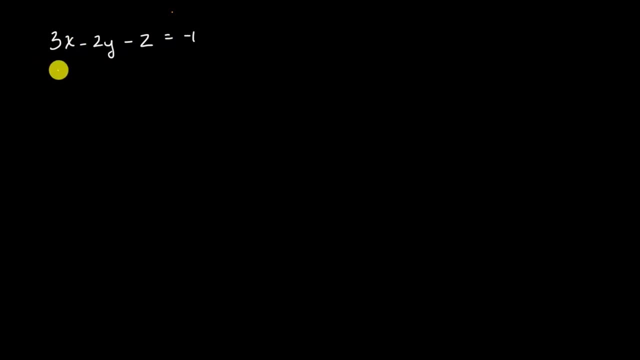 That's one equation, And in three dimensions this would represent a plane. And then I have another one: Two x plus five, y plus z is equal to zero. That would represent another plane. Now, if you had two non-parallel planes? 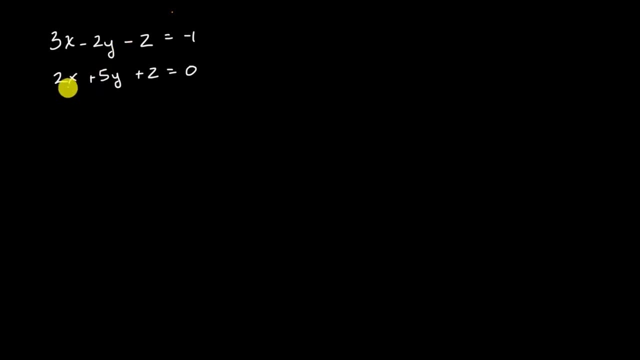 they would intersect each other and form a line. But then if we have a fourth plane, so let me write that as negative, four x minus y is equal to eight. it's possible- not always going to be the case, but it's possible- that they will all intersect. 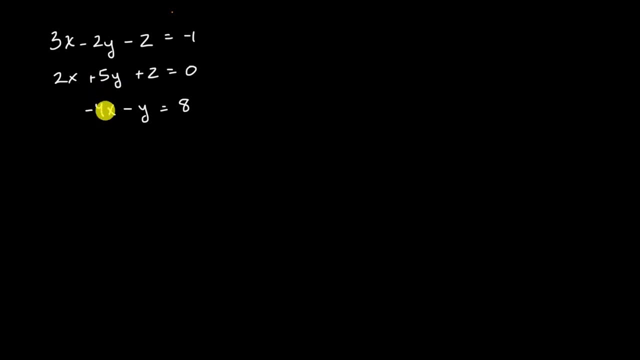 in exactly one x, y, z coordinate, And so in other videos we talk about solving systems of equations like this with three equations and three unknowns. Now what I wanna do in this video is connect this idea to the notion of matrices and matrix multiplication. 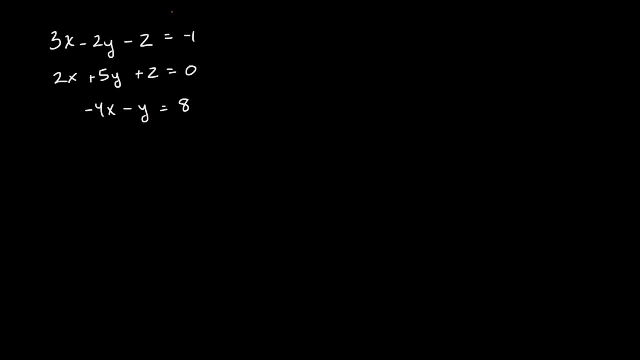 which we've already reviewed in other videos. So we can think of this exact same problem in the following way: If we take all of the coefficients and we create a three by three matrix with them, So let me do that. So, for example, let me get all of the x coefficients. 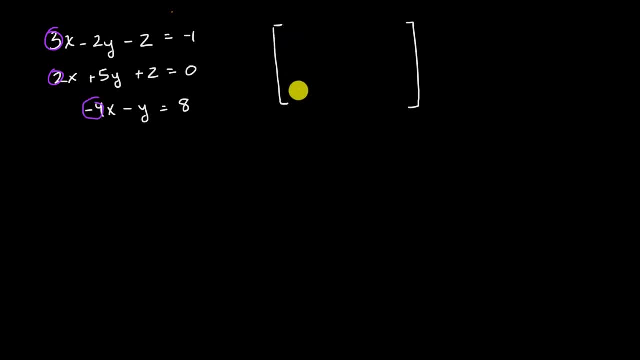 a three, a two and a negative four. And I'll put it in this first column here: Three, two and negative four. Let me get all the y coefficients: Negative two, five and essentially a negative one: Negative two, five and a negative one. 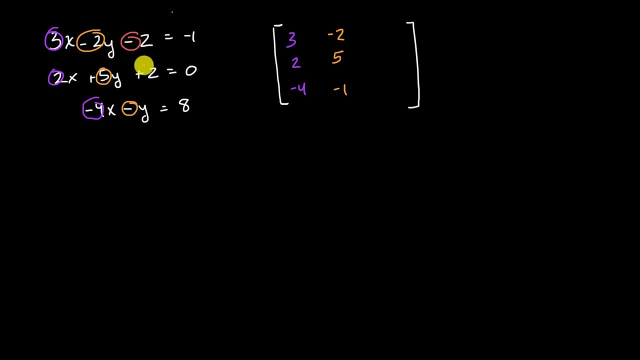 And then, last but not least, all the coefficients on the z's: A negative one, a plus one, and then there's implicitly a zero z here you can't see it. So it would be negative one plus one and then a zero. 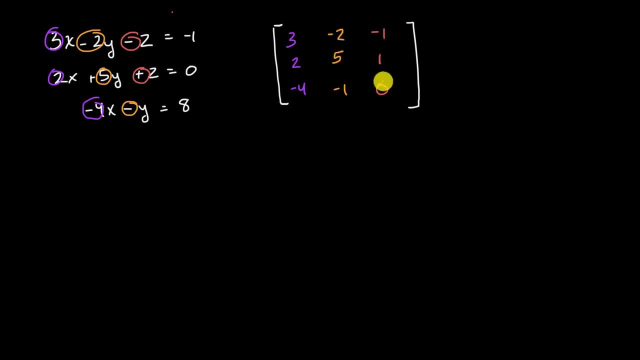 So these are the coefficients on x in purple, on y in yellow and in, I guess, salmon color. for the z's right over here, If we said that that is going to be multiplied by a three-dimensional vector, that is, I guess we could say, unknown- x, y and z. 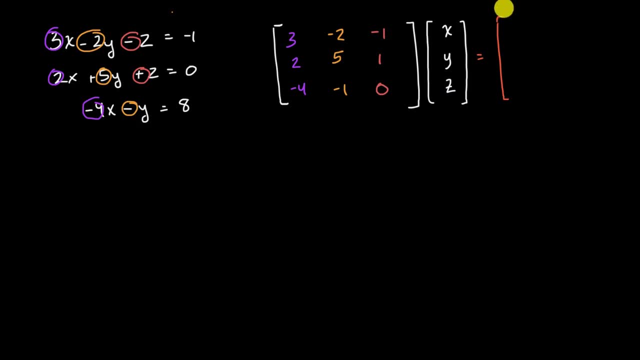 that is going to be equal to a second three-dimensional vector, which we do know, And that's negative one, zero and eight. And I know there's a lot of things going on in your brain right now. You're like Sal, this looks somewhat magical. 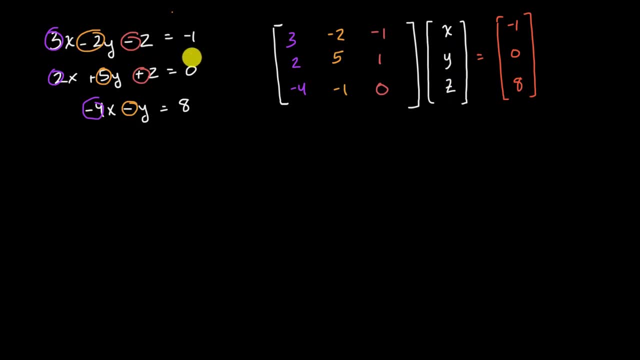 You just took the coefficients. put the x, y, z's here. put the right-hand sides of the equal sign, in this case the size that didn't have the variables on it. put it over here. does this actually make sense? 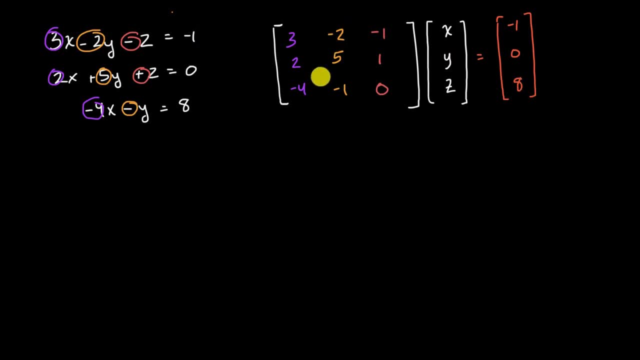 Does this actually work? And to validate that, let's actually multiply out the left-hand side of this equation right over here. So in other videos we've talked about multiplying a three-by-three matrix times a, in this case a three-by-one matrix. 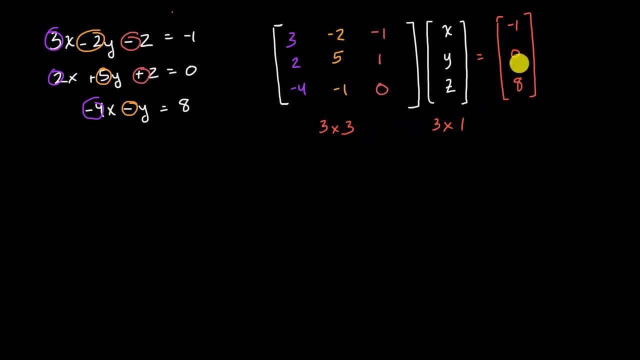 And this is going to actually give us a three-by-one matrix. So that's looking good already, And the reason why we know that is these two have to match in order for the multiplication to even be defined. And then the dimensions of the product. 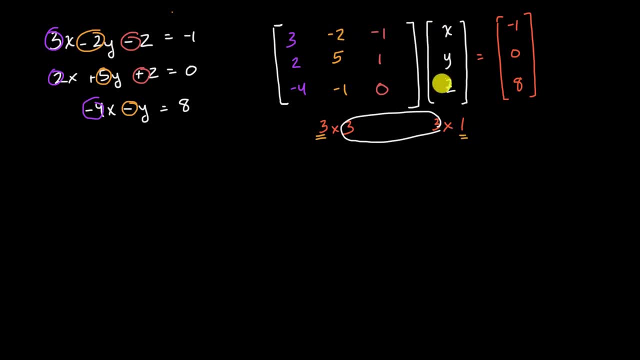 are going to be three-by-one, But let's actually multiply things out. Well, we know one way to construct this. I'm just gonna focus on the left-hand side here- is to say, all right, let's essentially take this row. 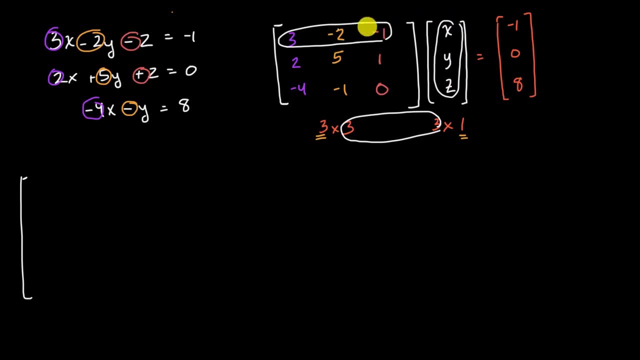 and this column and then take the sum of the product of the corresponding terms. I guess you could say So this is gonna be three times x, which is three x minus two times y minus two y, one times z minus one z, like that. 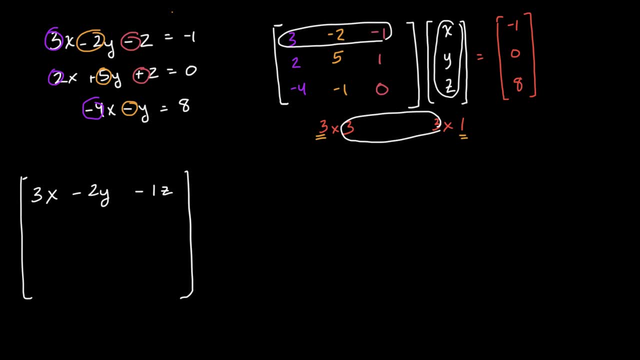 And then the next one. I'm going to take all of this business and multiply it by this column, So it's gonna be two times x- And this is just a review of multiplying matrices- plus five times y, plus five y, plus one times z plus one z. 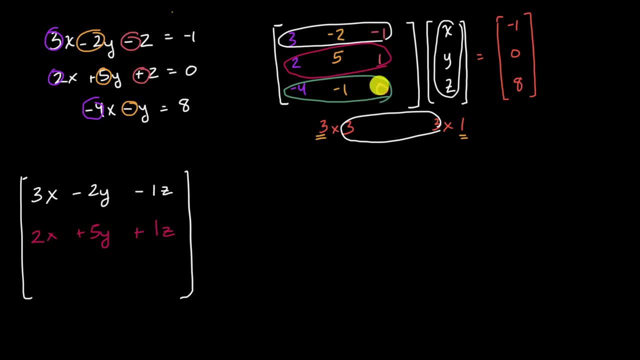 And then, last but not least, if I take this and I do the same thing with that column, it's gonna be negative four times x. negative four x minus one times y minus. I could just write minus y and then zero times z. 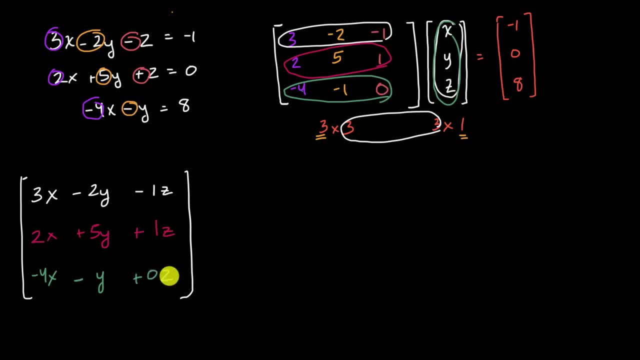 which I could write, if I want to or not write, but I could write it. let me just write it to make things clear. And so the product of what we have on the left-hand side is this right over here, And it might look like a three by three. 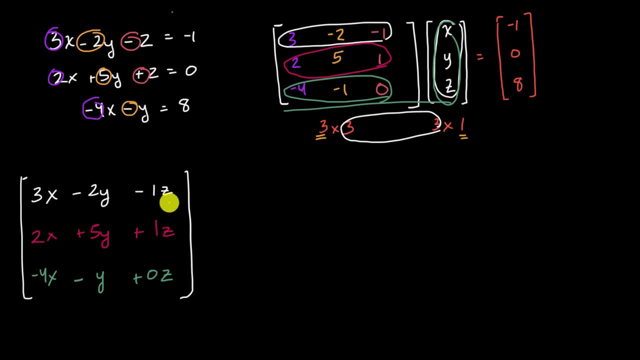 but it's actually a three by one here where this would, if you knew what x, y and z is. this is going to evaluate to some number. Likewise, this is going to evaluate to some other number and this is going to evaluate to another number. 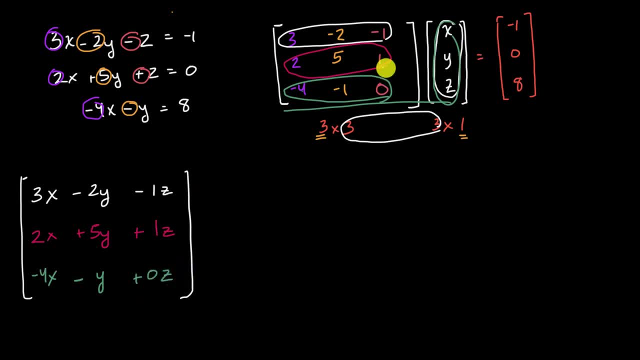 And we know from this- I guess you would say matrix vector, this matrix equation that we have set up, that this the left-hand side. this product needs to be equal to what we have on the right-hand side. It needs to be equal to negative one, zero and eight. 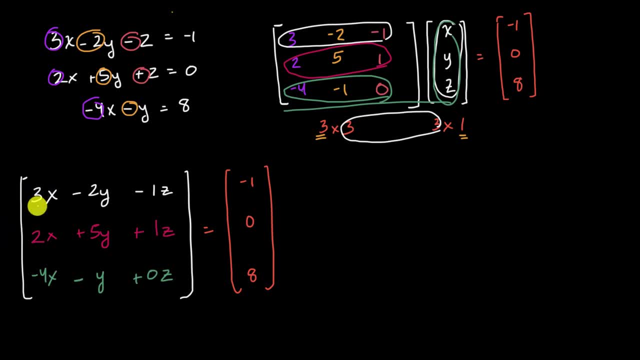 which means- and I think things might be connecting for you now- that this needs to be equal to that And that this needs to be equal to that And, last but not least, negative four X minus Y plus zero Z needs to be equal to eight. 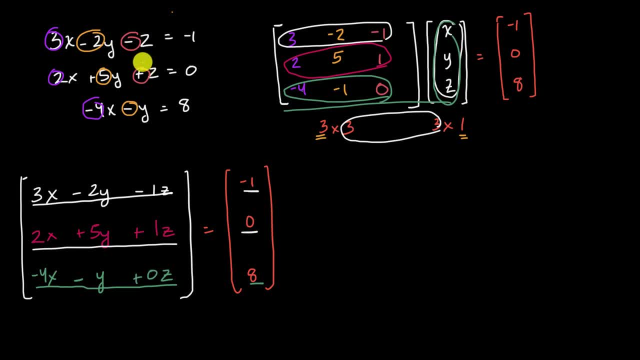 which is exactly what that original system of equations was telling us. Now I know well, there's still probably some things that are circulating in your mind. One question is: well, that's all nice. You found a different way of representing that. 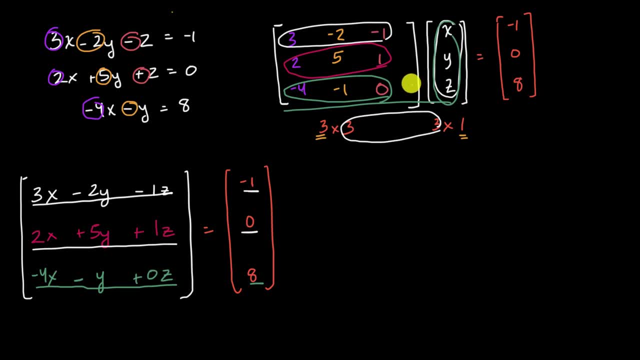 but how do does this introduce a new way of solving this? And the answer I'll give you for now is yes, it will lead to a new way of solving this because, if you think about it, we're taking the product of a matrix and a vector here. 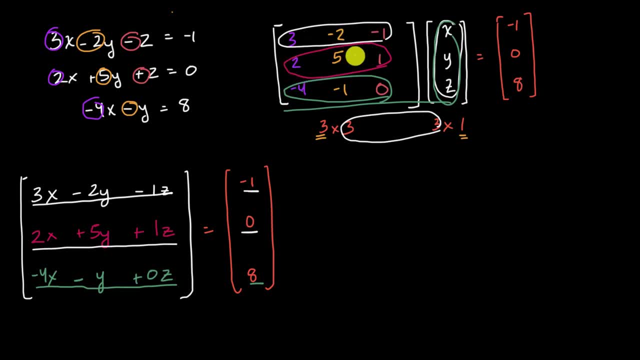 to get another vector. If there's some way to essentially unwind this matrix multiplication, then you might be able to do that, apply it to this vector on the right and then solve for this unknown vector here, And that's the way that things like a computer 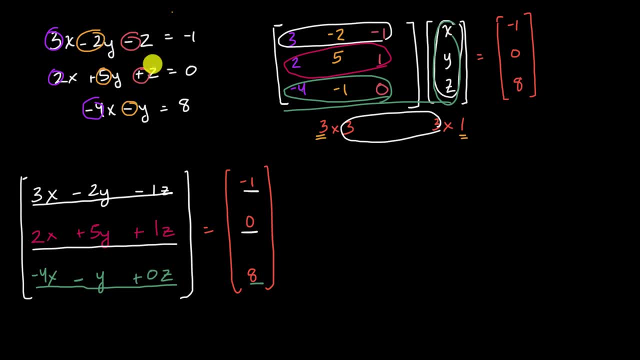 a lot of computer algorithms actually try to solve problems like this by representing them as matrices. Now another interesting thing just with the representation is it makes you think about the problem a little bit differently. You could view this as three planes and three dimensions.